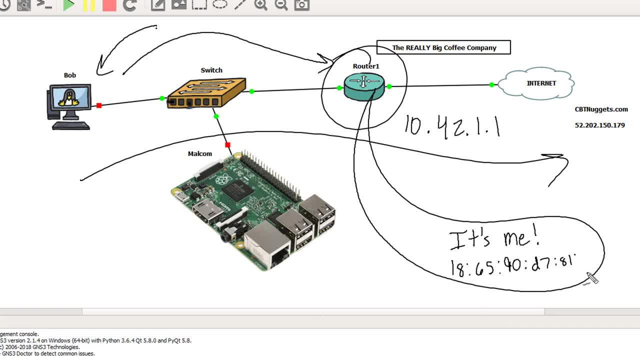 Here's my MAC address And then he replies with his MAC address. I always think back to when I first learned ARP, and it was watching Jeremy Chara's CSINT video. He always described it as like a dog barking like ARP, ARP, ARP, asking everyone. 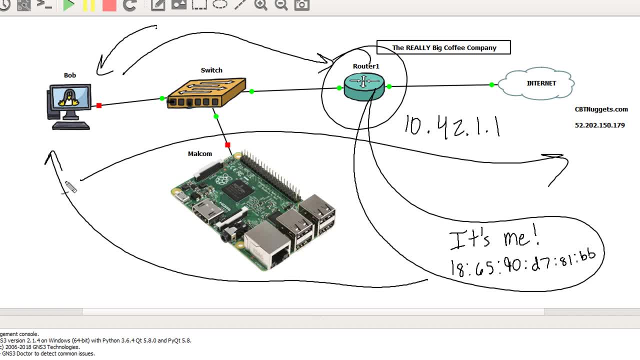 whose IP address this is. It's always stuck with me. So thank you, Jeremy. So we can see how Bob's computer found out how to reach the router. What we're going to do is slide Malcolm right in the middle there and kind of mess up that relationship, And of course we're going to use ARP spoofing or 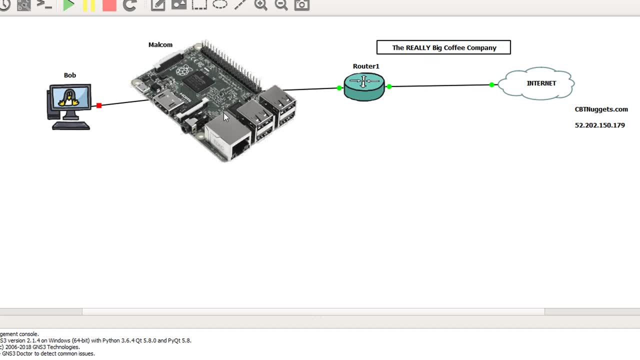 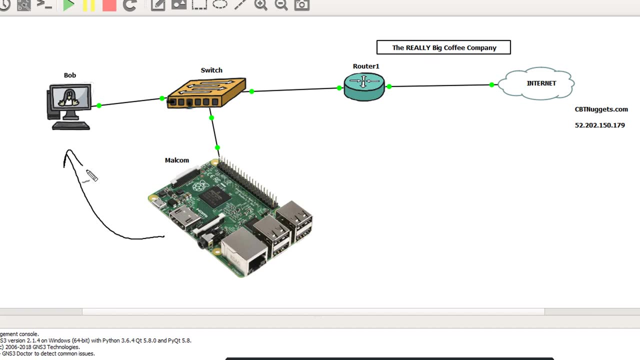 poisoning. So let's do it real quick. It's really cool, like stinking cool. Okay, so here's our mission with the ARP spoofing: I need to convince Bob that Malcolm is the router And I need to convince the router that Malcolm is. 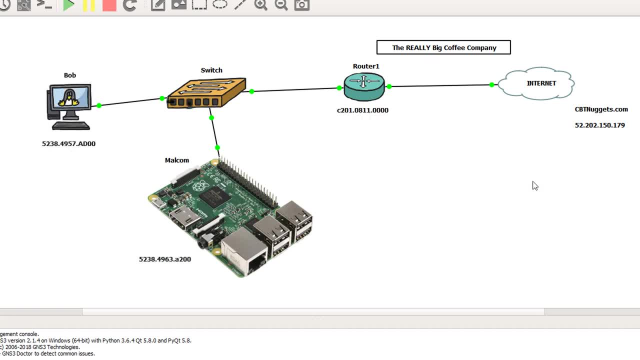 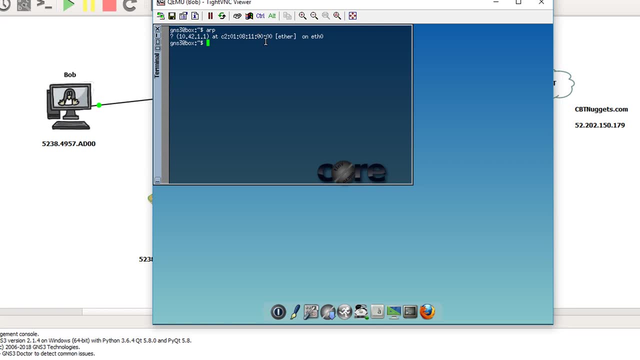 Bob. So let's get going. So first things first, let's see if Bob has the right ARP entry for router one. currently All right, so we see that right here for 1042.1.1.. He's got this MAC address. 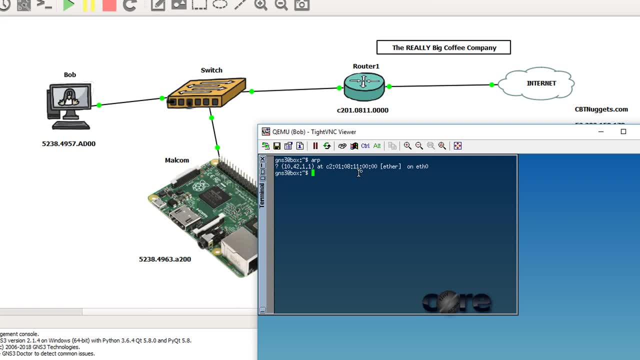 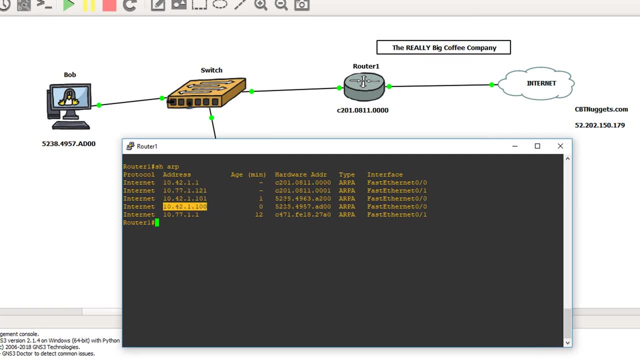 which does match up to router one. So he's good. right now Let's check router one. So I know the IP address of Bob is 1042.1.100.. And the hardware address which we have is right there. it matches up. So right now router one definitely knows the real Bob. 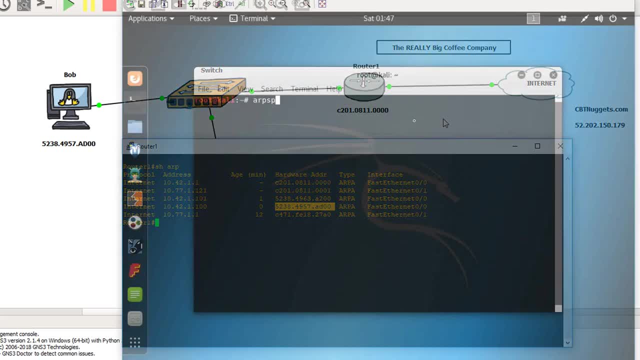 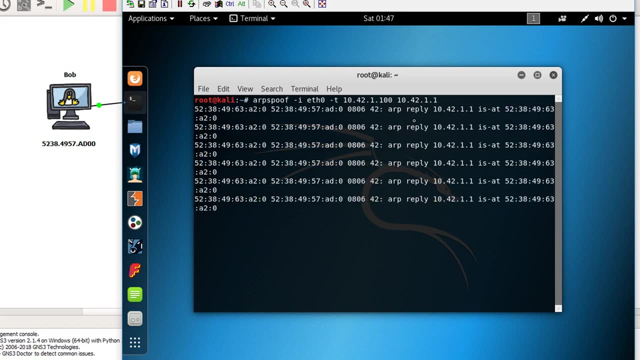 and Bob definitely knows the real router one. Let's mess that up, All right. so the first task we have is to tell Bob that we are the router. Let's go ahead and do that. So right now we are actively sending ARP replies to Bob saying, Hey, we are the router. Let's see if Bob believes us And would. 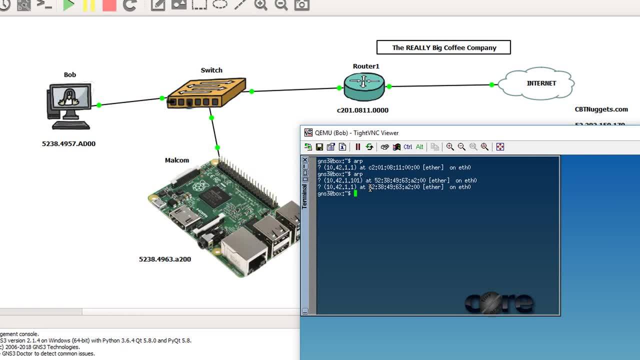 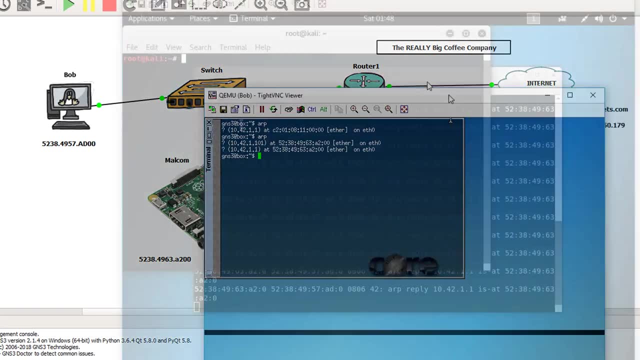 you look at that, The MAC address for 1042.1.1 is no longer matched up to the router one. It's now our little Malcolm here. Good job, Malcolm. Now let's do the same thing to the router. So now we're sending ARP replies to. 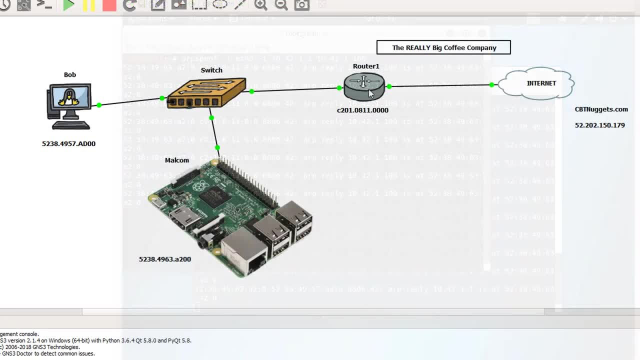 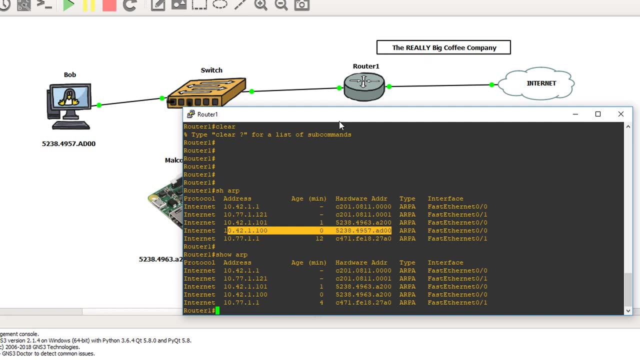 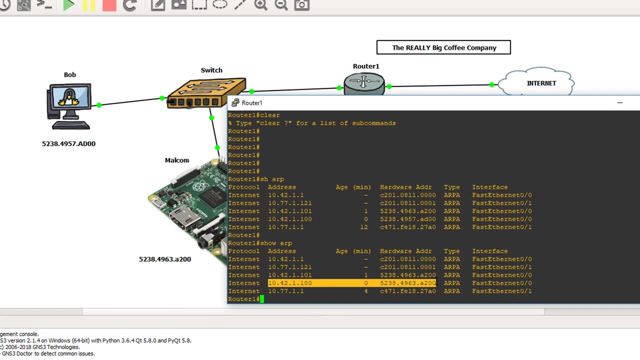 the router saying: Hey, Bob is actually Malcolm. So let's check the router and see if that worked. Aha, So you look at that now. So before it was matched up to our dear Bob, but now it's matched up to our Mr Malcolm here. So right now Bob believes that Malcolm is the router. The 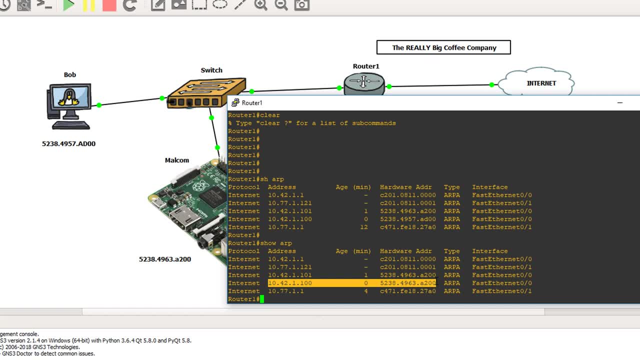 router believes that Malcolm is Bob. Malcolm is in the middle. Every packet is going through Malcolm. Now, a fun way to see this happening is there's two programs I want to use. One is going to show us all the websites that Bob will visit, and one will kind of pull up all the images from. 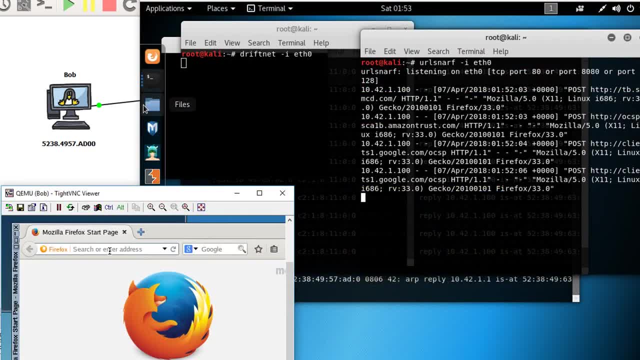 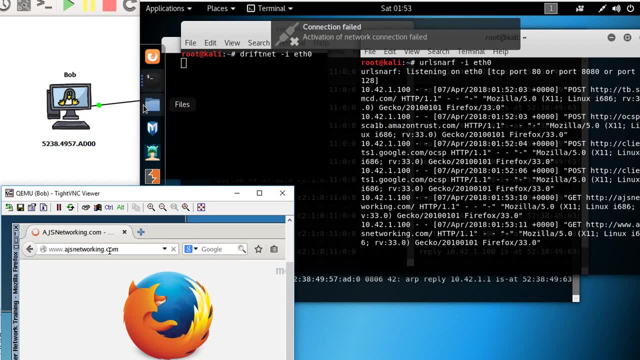 the websites he's going to. Let's go ahead and have fun with that real quick. So let's go to a website. Let's try Anthony Sequeira's website, ajsnetworkingcom. All right, so we're sniffing. 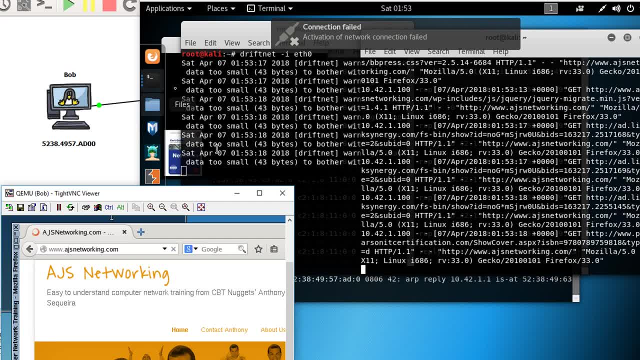 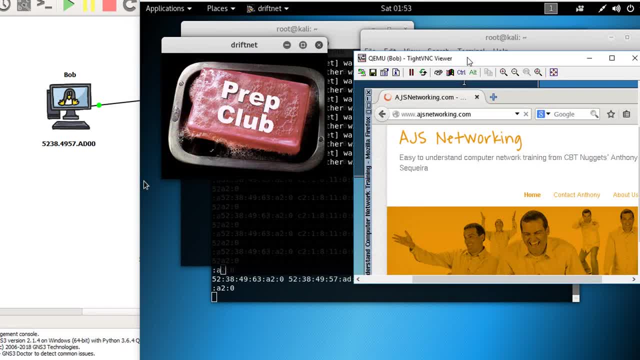 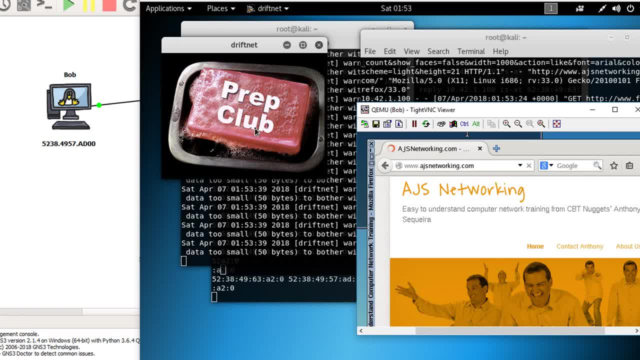 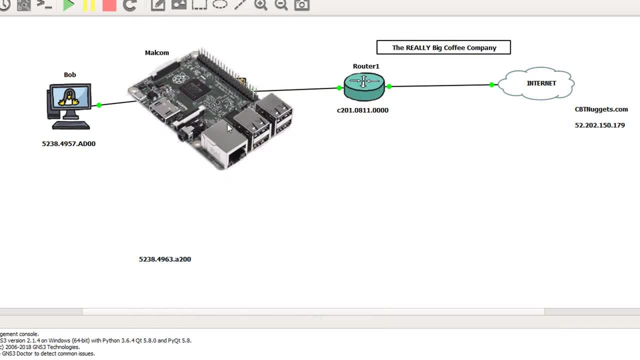 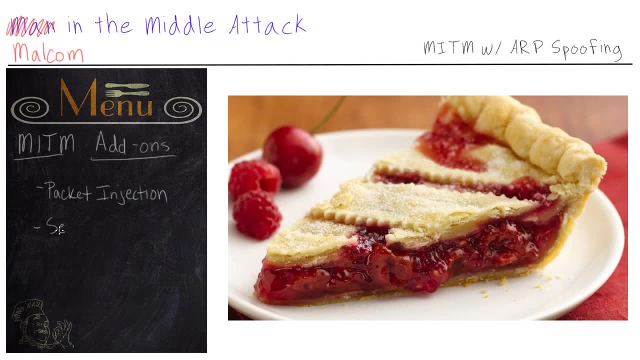 website he's going to and we can even see some pictures coming in. So right now we are the middleman. Everything Bob does. we see We have pretty much slid Malcolm right here, giving us complete control over all of Bob's internet traffic, Now that we have Malcolm in the middle. 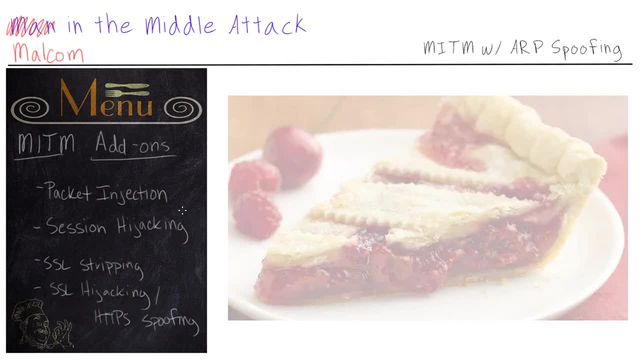 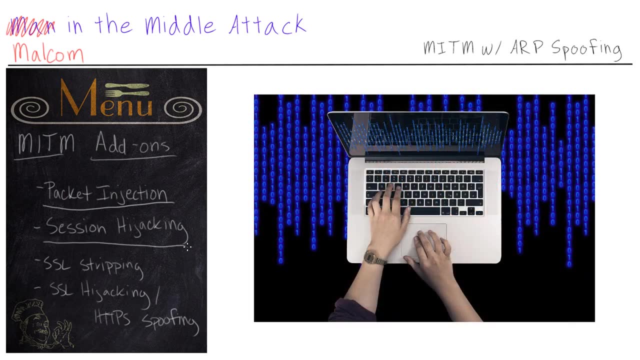 we can do so much more than just spy on Bob. We can do packet injection, where we actually craft malicious packets that we can send to Bob. Or we can do session hijacking Because, like most web applications, they'll use a temporary session token when a user logs into the website And 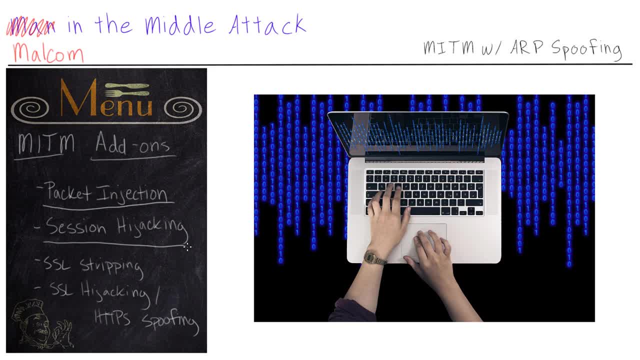 they'll use that token so the user doesn't have to keep logging in on every page. Well, as a man in the middle, Mr Malcolm can look at that token and use it himself and take actions on that site- So sites like banks- he can make a quick withdrawal or a quick transfer. Now, the majority of websites. 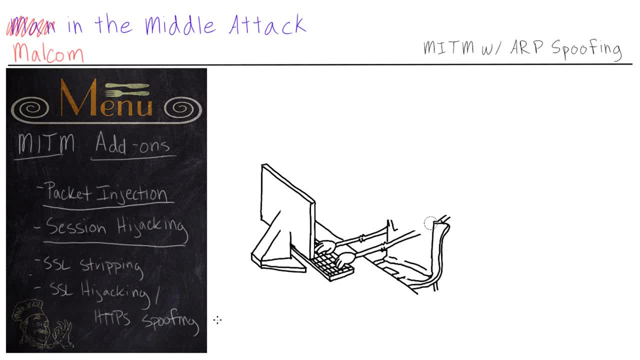 these days use SMS. So if you're using SMS, you can use SMS. So if you're using SMS, you can use SSL making the website secure. so we can't really see it, But we can do SSL stripping, forcing our local user, Bob, here to downgrade his session from HTTPS to HTTP So we can look at everything And